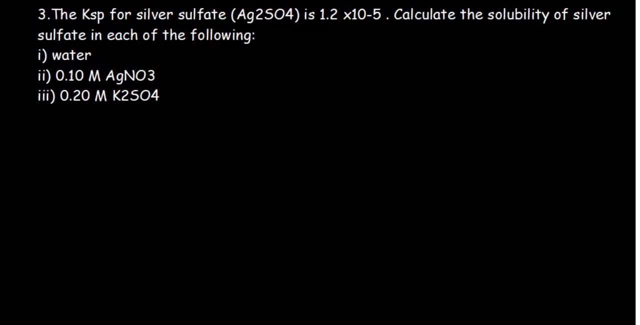 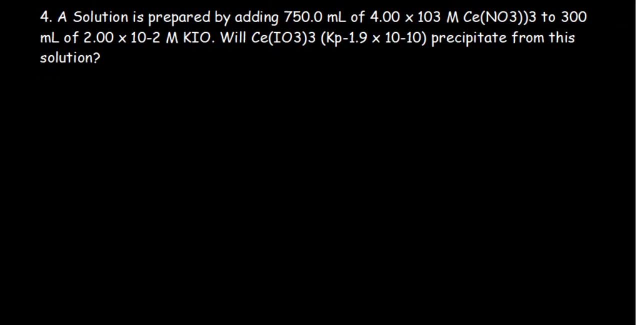 Question four is now focusing on precipitation. So when do we decide, or how do we know there's going to be precipitation, So we'll have to use what we call the Q Again, it's what we were talking about: the Ksp in this very case. 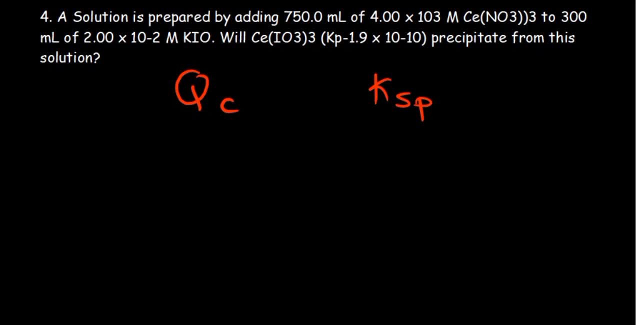 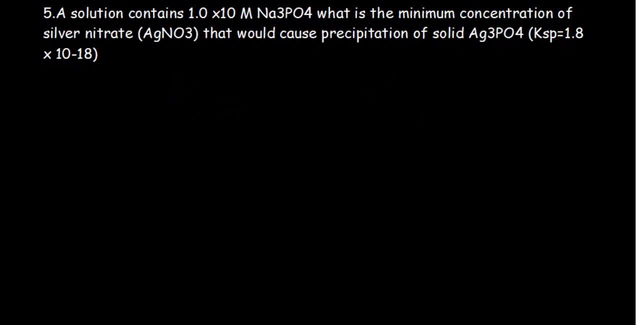 Okay, so from there again. this is another question on precipitation. Question six is almost dealing with precipitation, except we're trying to determine the concentrations at equilibrium. Question seven is: So we're focusing on determining the pH. So these are some of the things that we're going to cover in this tutorial. 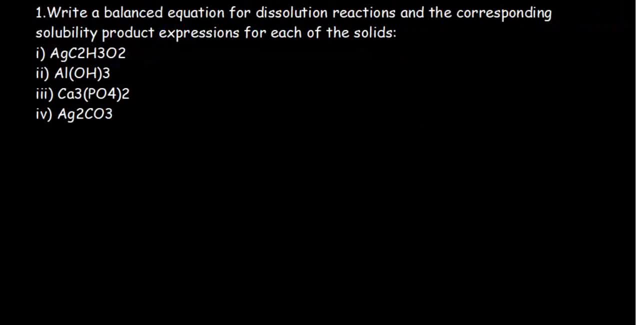 Okay, so basically, what is solubility equilibrium? What we deal with under the solubility equilibrium. So solubility equilibrium is basically a type of dynamic equilibrium that exists when we have a chemical compound that is in solid state and then it gets to dissolve. 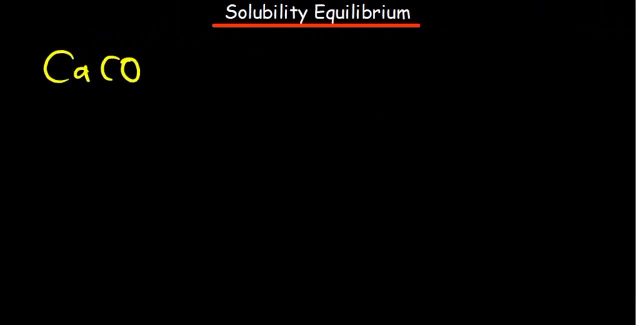 So the basic idea is: you have a solid, caustic and geosolubilistic. So you have a solid and a caustic and geosolubilistic. You're getting a solubility equilibrium, calcium carbonate, which is in in solid state. so when you get to dissolve this, let's say in water, 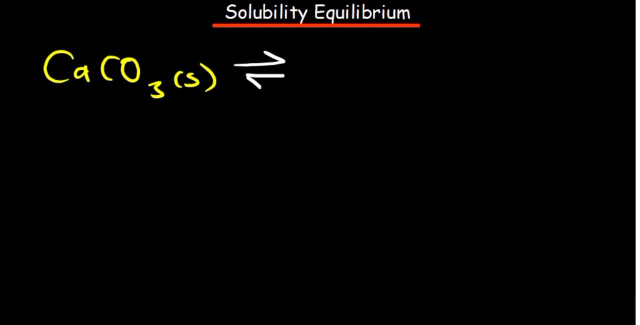 you expect that you're going to have production of what the ions, so of calcium. so we have calcium two plus, which is going to be in aqua states, and then we have carbonates as well, which is also going to be in aqua states, of course. that is two minus. 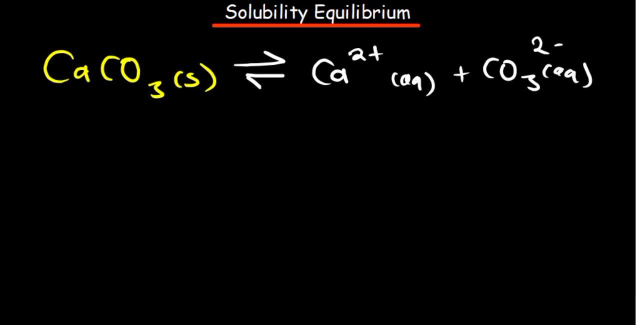 so so it could be basically is giving us. it's the chemicalilibrium where we have a solid and the solid is partially soluble and then so especially soluble. so we are going to see that in our solution there will still be a solid that is going to be present as well as 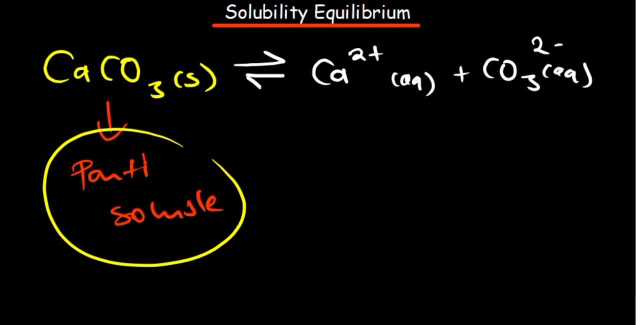 soldiers are also going to be present. so now that would mean that the rate at which the bare laboratory becomes the problem at which we are destroying our advantages, the brain needs to reactions occurring is equivalent to a forward reaction. so that is solubility equilibrium. we have a partially soluble solid being dissolved and then, when it 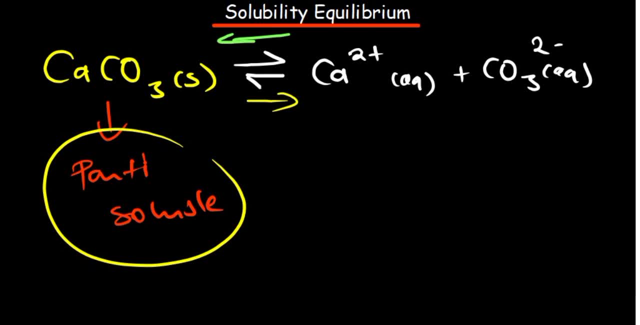 reaches dynamic equilibrium. we refer to that as solubility equilibrium. okay, so now that we know what solubility equilibrium is, let us try to understand what solubility is. what is solubility? so when you talk about solubility, you are just trying to estimate, or we can consider solubility to be the 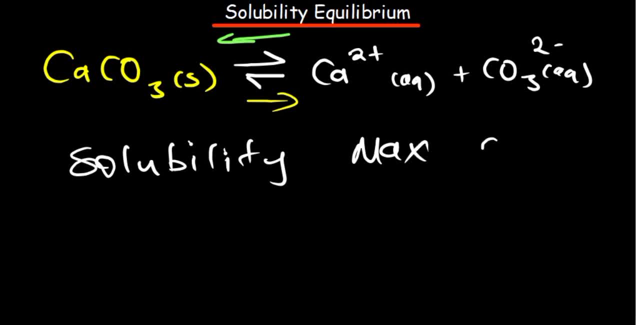 maximum, the maximum amount of solute that can do what that is going to dissolve. so surability is the maximum concentration of solid that can be dissolved in the solvent that we have. okay, so this is the basic idea about solubility, equilibrium, and what we can talk about is- we can even try to look at the same. 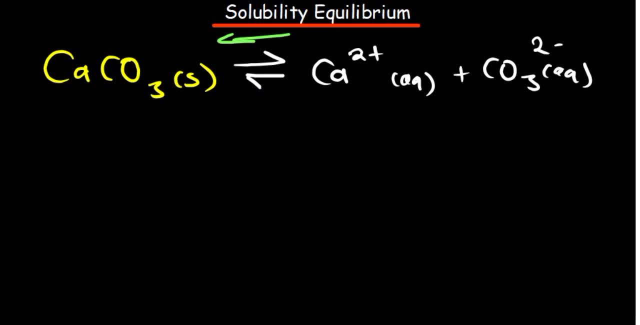 equation that I've given as an example and understand the way. the case P depends on what we have. so if we've done chemical equilibrium, we do understand that solids do not appear in the K expressions. so in this case our K is referred to as the KSP, which stands for solubility products. okay, so basically, if 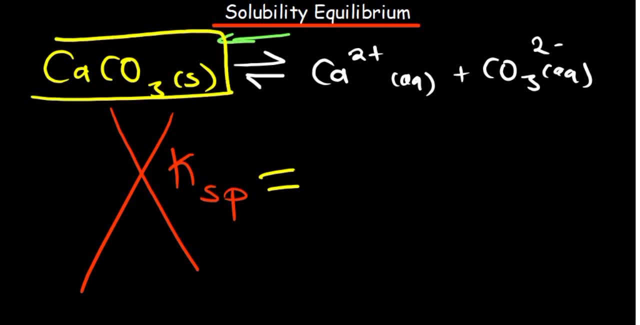 you look at what we have, our reactant is a solid, so we only expect our ions on the right hand side to appear in the KSP expression, just like we did under chemical equilibrium. so therefore, we're going to have calcium 2 plus and then carbonate 2 minus. so these are the ones that are now representing the KSP. 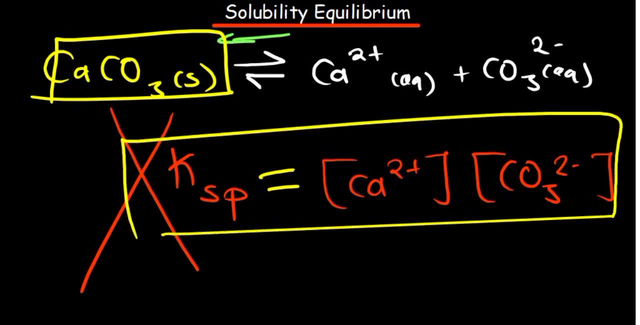 expression. okay, so understand later as we look at some more complex questions on how we get to to simplify this. okay, so we'll start your first question. the first question says: write a balanced equation for dissolution reactions and the corresponding solubility products expressions for each of the solids. so just like we know when. 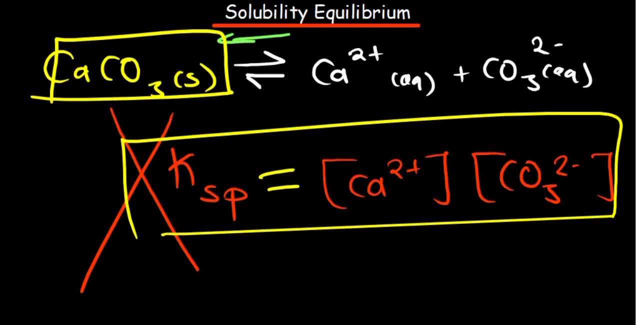 I talking about solubility equilibrium. what we are talking about are solids. so all these are solubility equilibrium. so we are talking about the solubility equilibrium. what we are talking about are solids, so obvious are. so it states, as the question tells us. so i'll start with the first one. 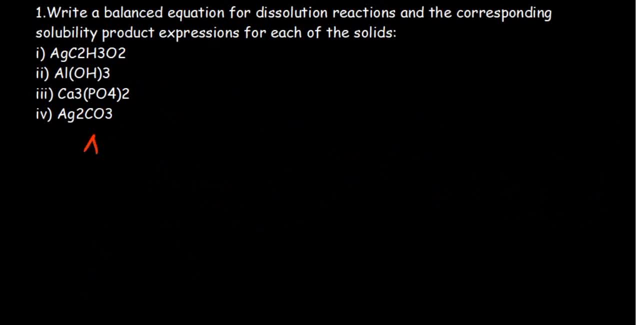 so if i got the first one, what we have is silver, and then we have six, two, eight, three or two. so that is solid. so to show that this is at one point going to reach equilibrium, we'll use those two arrows and then we'll split this into the ions. so the only iron that we can clearly see is silver. 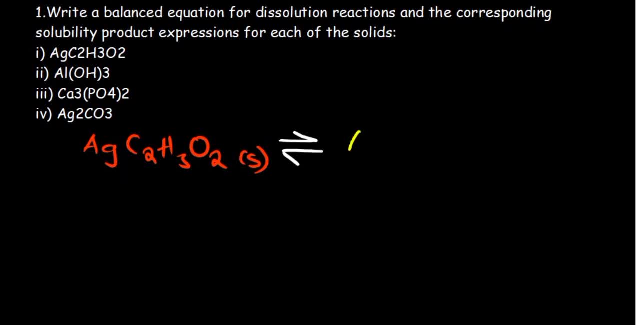 okay, so our silver, which is ag plus, and then the other substance as well. right, it is, it is okay. so this is what we have in our equation. so this is a balance. is it balanced? so it is, so we've answered. the first part of the question says: write a balanced equation for dissolution reaction. 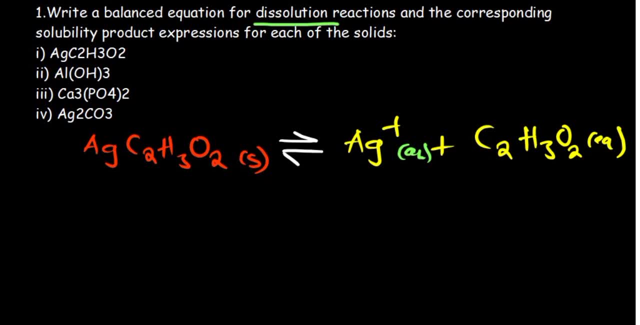 and then we need to write the ksp expression. so the ksp expression for the sake of our understanding. in this case i'm going to use the ice table and then, on the other examples, i'm not using the ice table because you're going to get the concept so solid, does not? 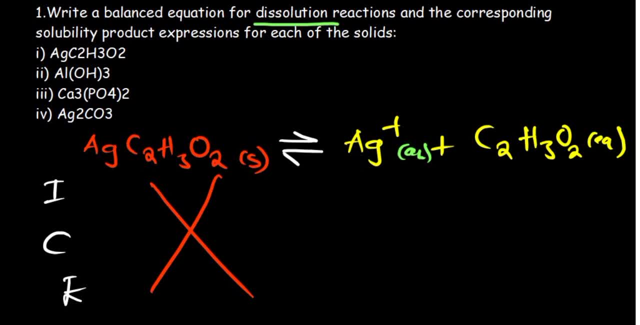 appear in the k expressions. and then, for our silver, we didn't have any initial concentration, knowing that we started with a solid, so i'll put zero, zero. and then, just like we did under chemical equilibrium, we're going to use a variable. in this case we'll go for x. so positive x and positive x. 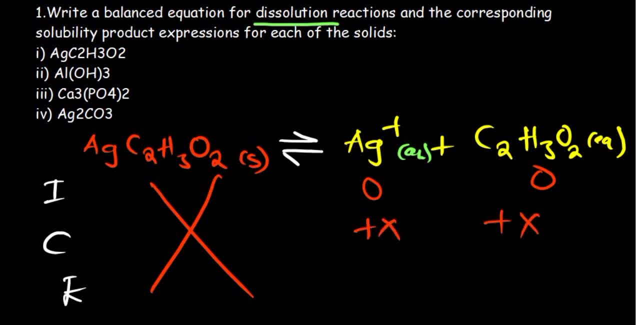 of course this is affected by the coefficients. so if we add the two there, it is going to be 2x, but in this case we just have ones as a coefficient, so it will just be plus x, which tells us to say that as the reaction progresses, we expect that there should be an increase in the concentration of 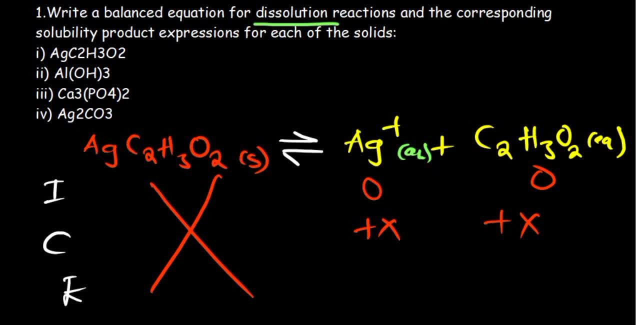 our products, meaning that part of the solid is going to be dissolving. okay. so therefore, in this case, our equilibrium concentrations will just be the changes, because zero plus x will remain the same. so therefore, our ksp expression, knowing that is dependent on the equilibrium concentrations, is just going to be x times x, which is going to give us x squared, okay. 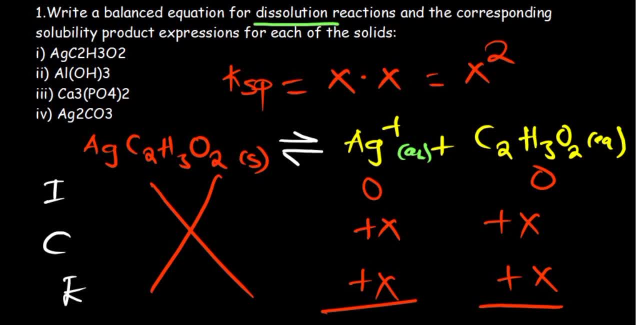 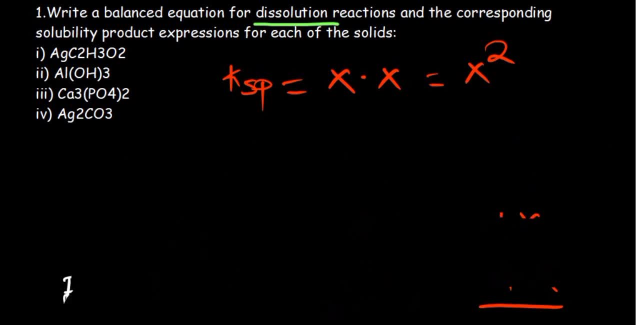 so if you want to present your answer in a more organized manner, what can you do? you can decide to show the same ions that we are breaking down. let me just bring that back so you can just put it as case and just put the same answer. okay, so now, if you have this space x, you'll have to. 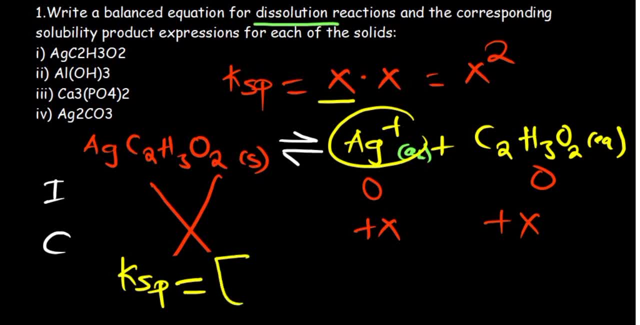 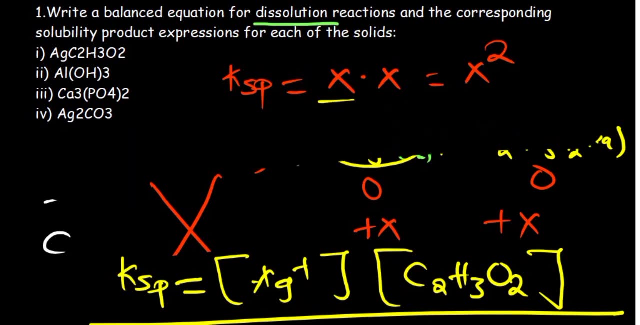 get this, guys of the fourth dimension of this Kahwa, the third dimension of this, so stay tuned. i hope you get that, looking at your analysis of the ceremony, is equal to two psi x long suised and three pr米 what. you know that the first x is denoting the silver, so you can just put the silver there. i on and then multiply against the other one there, so that is also one on the same. that's what we have, okay. so therefore, as he gets to look at the other, they have a JD that we're given. they're going to be very easy. so if you're very minimum, i can give you two pi the DIiminganti. 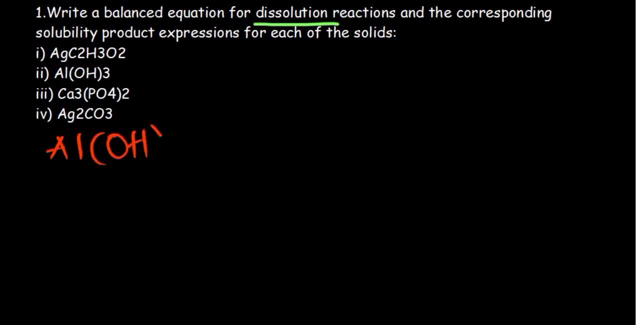 if you have aluminium hydroxide, so how do you know how to balance this? so if you have aluminium and then you have hydroxide, so what? the basic idea is this: three is going to go there and then what is there is going to to go there. so you know that metals are going to be positives. 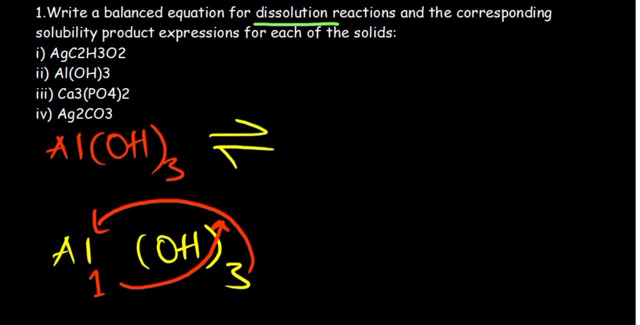 positive ions, and then these others are going to be negative. so therefore, in this case, aluminium is going to be aluminium three plus, and then we have hydroxide. of course, hydroxide is a common one, so it's going to have a negative there. now, is it balanced? 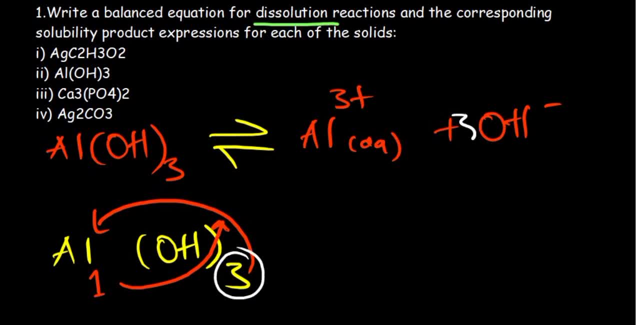 no, we had three hydroxide there, so put three there, and then aluminium will just remain the same. so of course that is in solid state. these are in aqua states. so therefore in our ksp expression we don't expect to show the aluminium hydroxide. 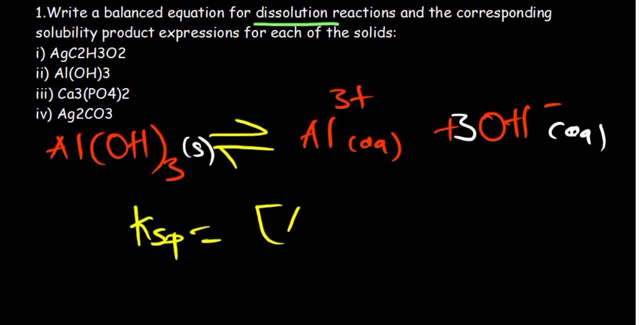 we'll just go for the ions on our right hand side. so now, in this case, you're going to pay more attention to what i'm going to show. so if we are going to write our ice table in this example for a change for the hydroxide, is because going to be plus 3x, this one is just going to be plus. 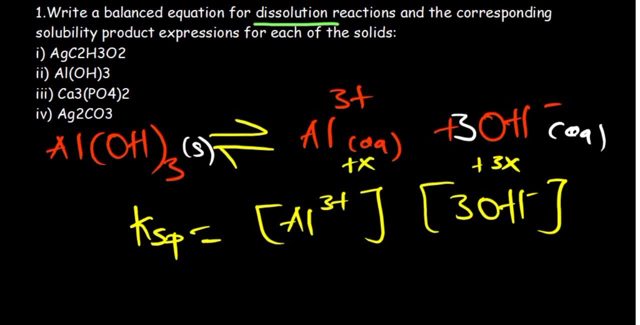 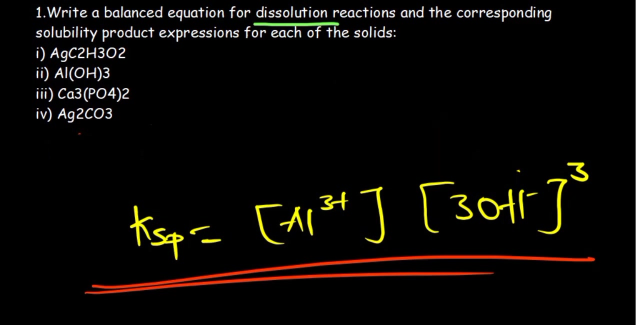 x. so therefore, that's why i'm putting three hydroxide and, of course, what we know from our chemical equilibrium means every time we are doing that, we get to raise everything to their coefficients. so therefore, this is going to be to the third power. so therefore, that is our ksp expression, of course in respect to the solids that we have been produced. 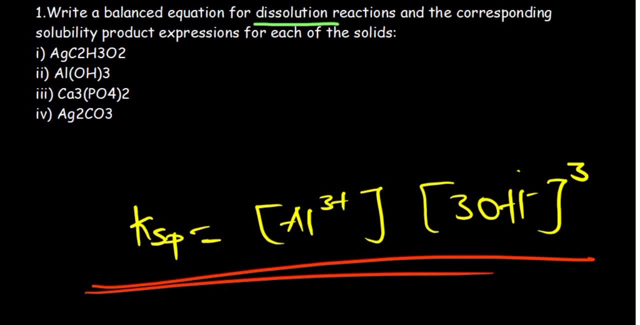 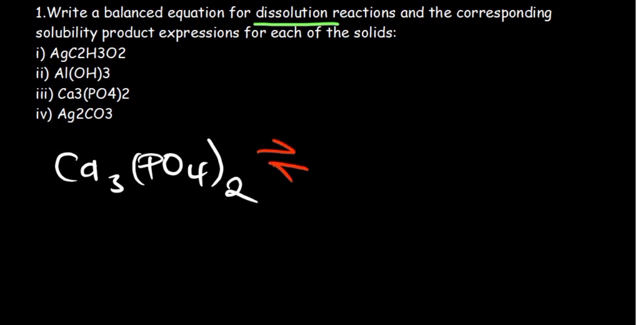 for the second one. so feel free to try out the the next two. okay, so of course, if we go to to the next one, we have calcium three and then we have po4 two. so this is going to be the last one i'm going to do. of course, this is in solid state. so now, just like we said, this is supposed to. 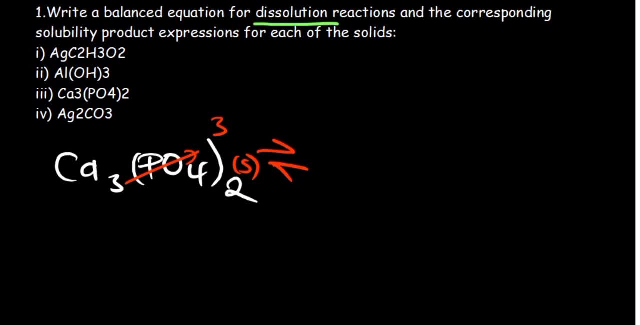 exchange. so therefore the three will go there to the three minus, the two go there to be two plus, because metals they carry positive charge, positive ions. okay, so three minus two plus. so we have calcium two plus plus po4, which is now three minus. now for us to balance, we need to look. 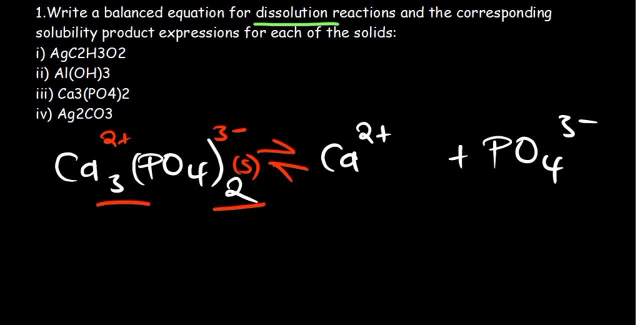 at the sub. yeah, we need to look at the sub coefficient that we have there- subscripts, sorry. so we have for calcium we have a three, and then for p or four we have two. so in this case we've balanced our ions in our equation. so all these are in our quarters. six plus two is four, so now the 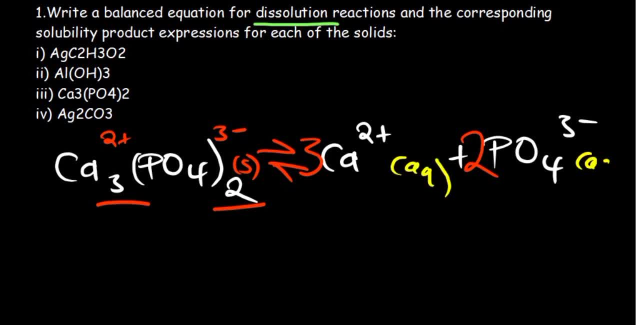 third one i'm going to do is we're going to change the two and the next one is the three. so we're going to aqua states. they were important and therefore our ksp expression is therefore going to be equivalent to our calcium. of course i'll put a three, so three calcium, two plus ions. 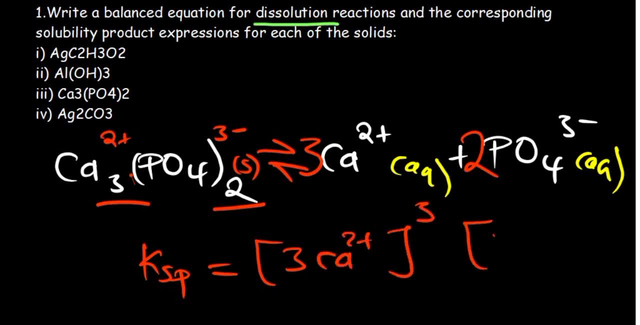 raised to power three again. two p of four should also be raised to power two from our rules under chemical equilibrium. so this is the ksp expression for the third one, and that is how you get to give the ksp expression in respect to the solids that are being produced. okay, question two. question two. 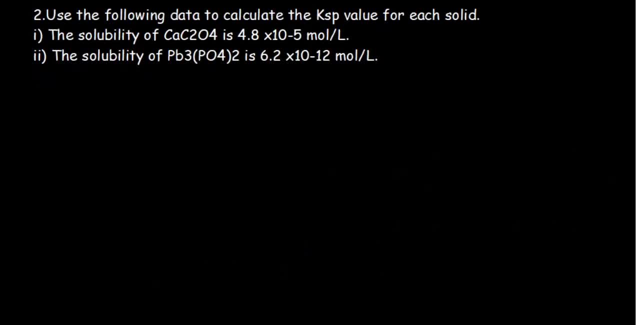 we are asked to use the data to calculate the ksp value for a solid. so the first thing that we would want to do first of all is gets to write the dissolution reaction, which is very, very important. so if i look at the first one, which says calcium, 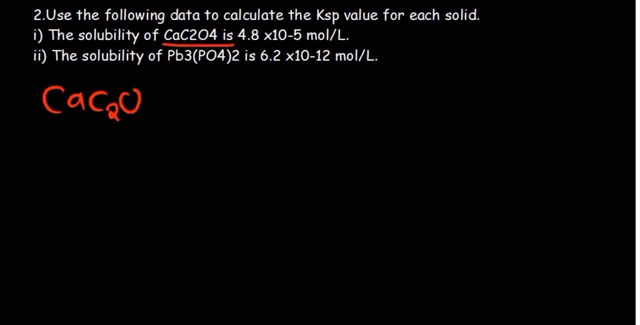 and then we have c two of four as our solid. okay, so what do you get to do there? so if you get to write your equation there, you expect to have. now the funny part is, you do know that calcium of course comes with a charge of what? two plus right, and then the fact that this is separate from calcium we expect to. 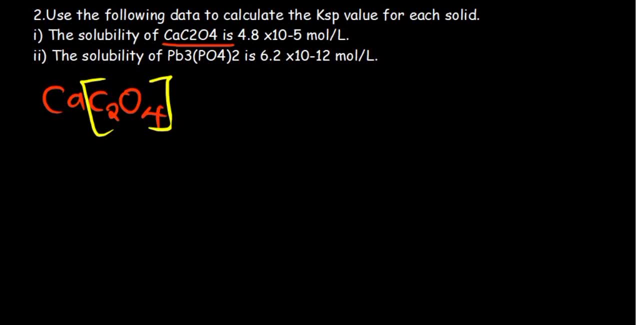 have a two outside right. so let's try to do that, so we can have calcium and then we can factorize it to that, so that you have carbon dioxide in the brackets and then you manage it too. it makes more sense in that case, and that's what we're going to. 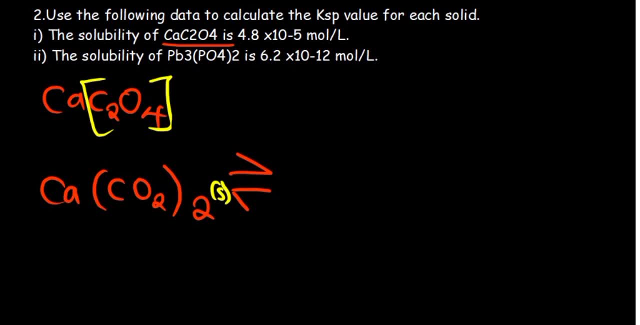 do, which still, which proves to say we are going to have calcium ion reacting with carbon dioxide, right, yeah, so therefore we have calcium two plus states with carbon dioxide in aqua states, And then what we have? we can have these two on the carbon dioxide path. 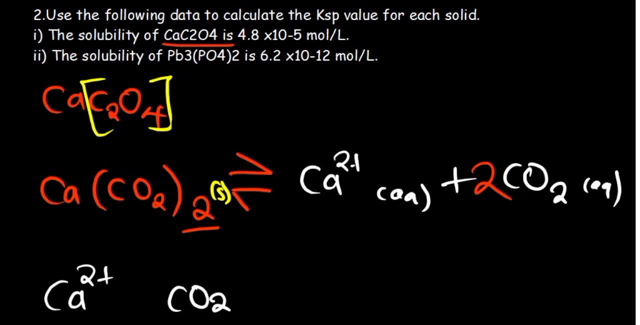 So this is basically very, very important for us to show: What can we say now? What can we say So? we've balanced our equation. Now the Ksp expression is going to be what? So the Ksp expression is going to be dependent on this. 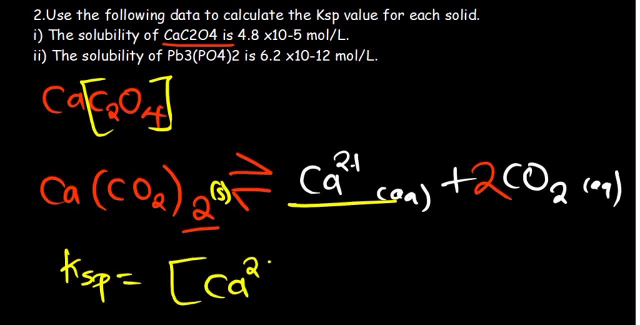 So we have calcium 2 plus the power 1, and then we have carbon dioxide, the power 2.. Now, one point that I didn't make is Solubility. basically, is going to be the same for our solids that we have. 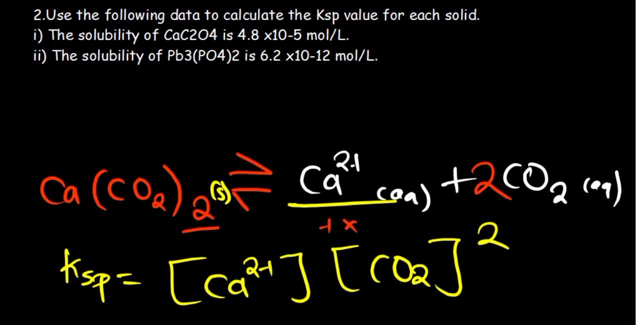 So on the part of our change, this is plus x, that is plus 2x if we are going to write our ice table. So you can clearly see that the value of x is what Is 1 and the same. So in fact in our Ksp expression I'm supposed to put a 2 on the carbon dioxide path, because 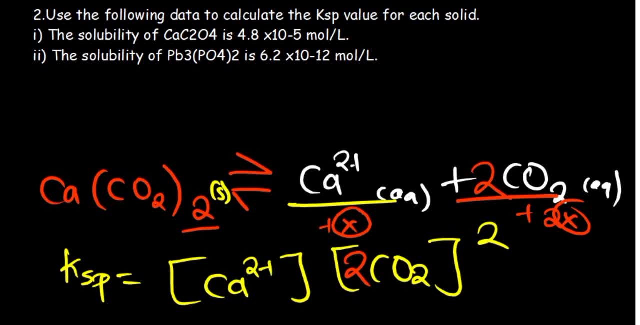 of our equation. And then what I'm going to do is I'm just going to put the values of x Directly, Directly, Directly. So for calcium we just have x, And then for 2 carbon dioxide I'm going to put 2x. that's our change, and then it's supposed. 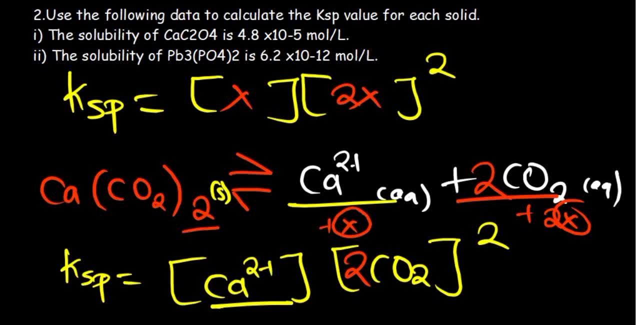 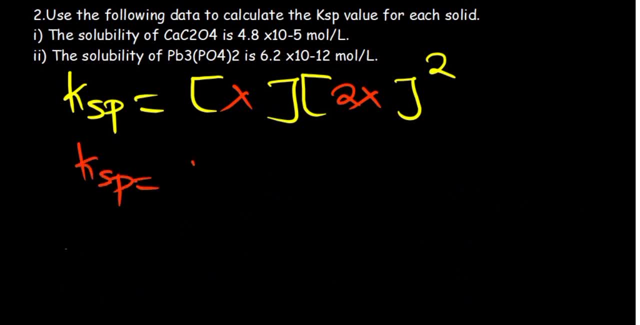 to be raised to the power 2 again. So, as we get to simplify that, what do we have? So our Ksp expression, therefore, is going to be equal to 2x. 2x squared is the same as 4x squared. 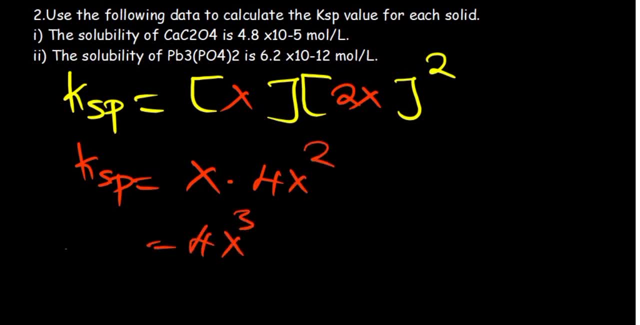 And then you have 4x squared to the power 3, so now the value of X is what we call the solubility. so in the question, we have given us what we've given us, a solubility, which is concentration, of course. so all you'd want to do is a substitute, the given. 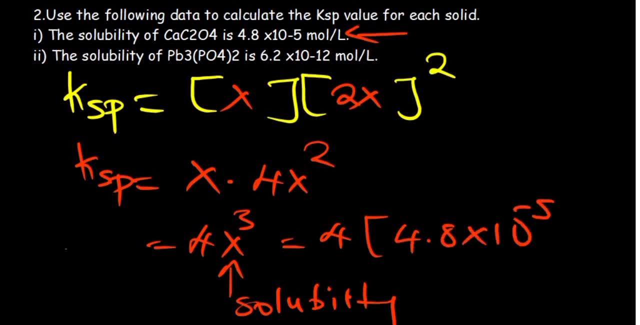 value 4.8 by 10 to power negative 5, and then we can now find the KSP. so grab your calculator: 4.8 by 10 to power negative 5, multiply by 4. so I'll repeat that again: 4.8 by 10 to power negative 5 should be first of. 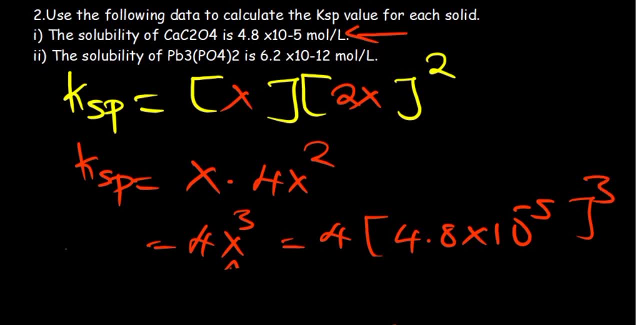 all is the third power. so the third power, and then from there we need to multiply it by 4. so what I'm getting is the 4.42 times 10 to the power, negative 13. so this is our KSP expression of value for the first part of the question, and then, of course, feel free to try out. 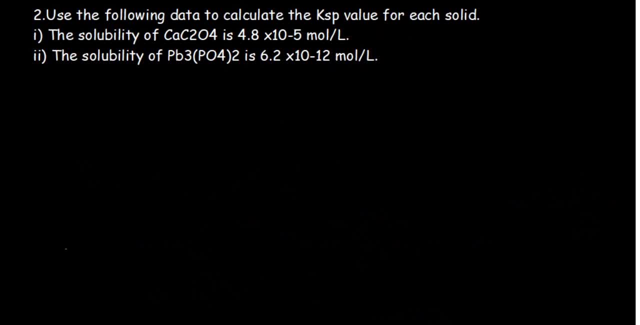 the second one, which is also almost one and the same, so PB 3, and then we have P of 4, 2 solid state. so what we expect to be our expression. so we have a 2 there. so the two is going to go on there on on the PB B there. 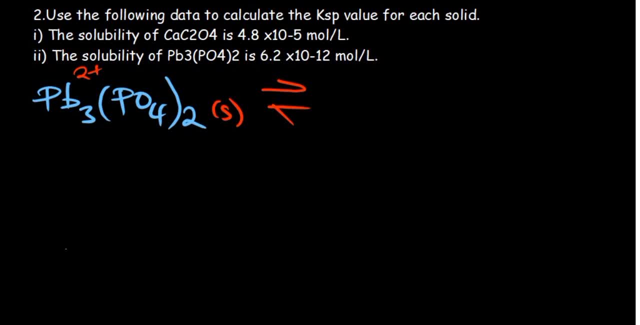 which is a yeah, and then the three is going to go this other side. ok, so PB is the red, so yeah, they don't matter. so, and then we have, but it's going to have a 2 plus. then we have phosphate, so this is going to have a. 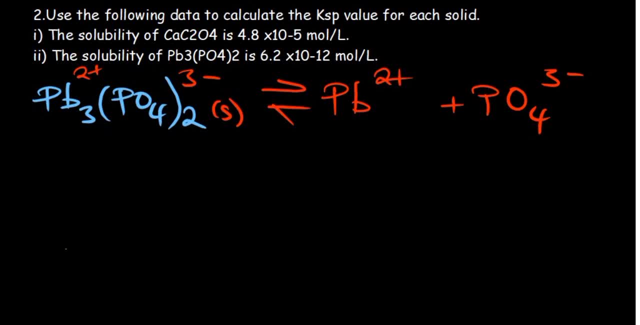 minus. and then, of course, the coefficients are going to depend on the subscripts. so what is a 3 and that is a 2 for a phosphate. so therefore, I'm going to use the I stable in this case, so that you can now maybe get it, in case you. 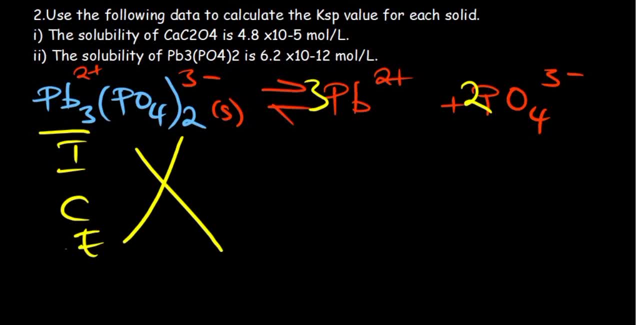 didn't get it from the first part, so sorries do not appear in the KSP expression. we didn't have any initial concentrations. according to the equations, the changes were 3x- 2x. this is dependent on the coefficients that we have. the equilibrium concentration is going to be given as the addition of the 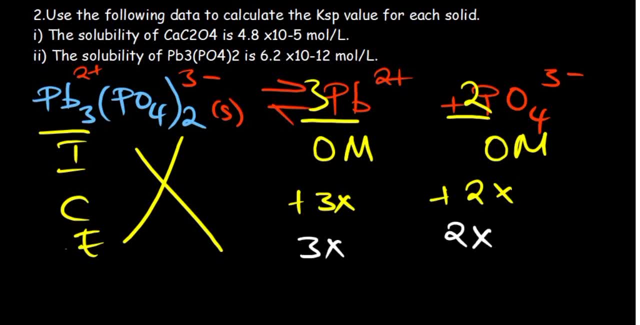 initial and the change, 3x and 2x respectively, and of course the KSP expressions, therefore going to be 3x, should be raised to a, such a metric coefficient, which is a 3 and then 2x, which is what should also be raised to a. 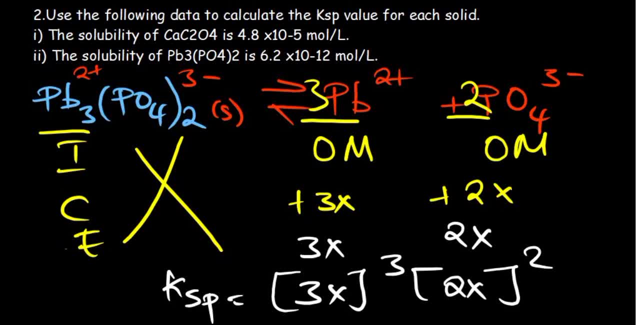 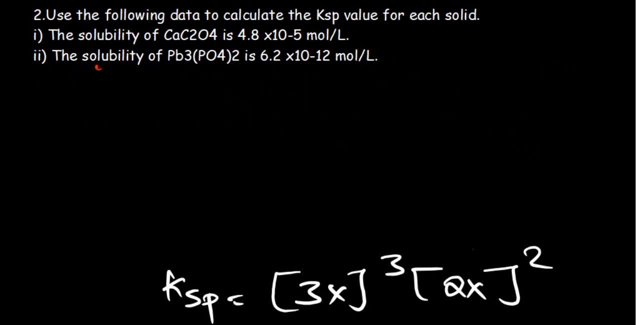 such a metric coefficient, which is also a 2, so you have your KSP expression in terms of X, and then you can now simplify. so my advice to you is, first of all, try to simplify everything in terms of X, so 3, the power 3 is, of course, going to be 27. 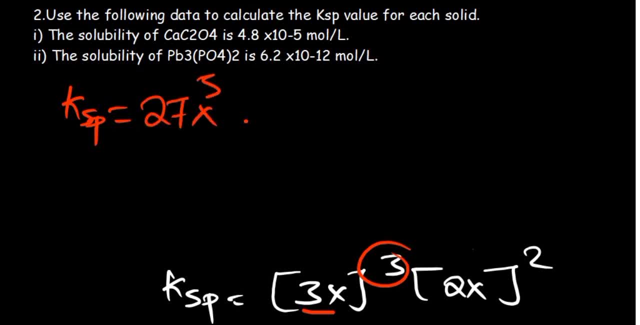 and then, of course, 2x squared is going to be like 4, if I'm not mistaken, 4x squared, and then, if you try to so 3, the power 3 again is 27. now 27 multiplied by the 6th power negative, 12. just 보시면, of course, you got a 4 from 1 0, 8. yeah. 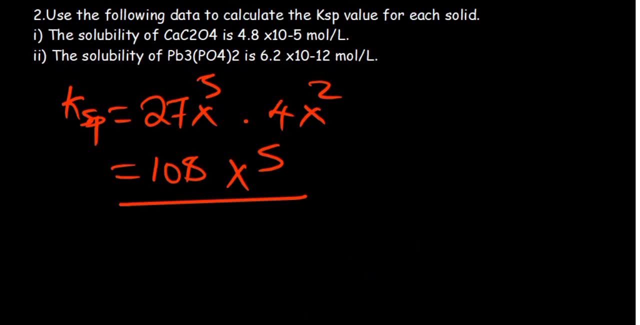 1 0 8, so one 0 8. X to power 5. let's CK expression you can now substitute in the equation that we have: X is denoting the solubility. so we just plug in 1 0 8 what Y by 6 points to. by 10 to power negative. 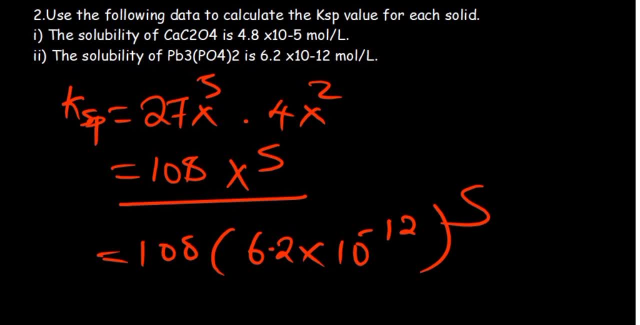 twelve right so of cost to the power 5, so 6.2. by 10 to the power negative 12, raised to the power 5, multiplied by 108, so approximately our value is 9.9 by 10 to the power negative 55. 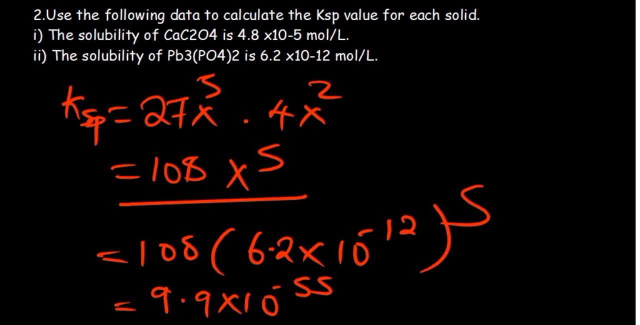 that's our KSP expression or our KSP value. that is moving on to the third question. it is basically the same from the second question. the only difference is we now have an initial. we've been given first of all the initial, the initial, what, the initial concentration of our solutes. 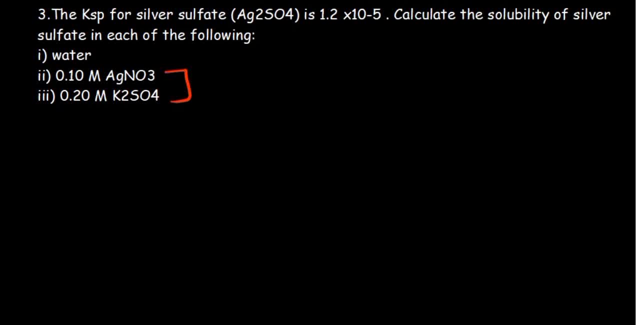 in the two last, yeah, in the two last questions. in the first one it is just pure water. so which is basically going to be under the same way we are from under in what the question 2, part 1 and 2. so Ag silver sulfate. 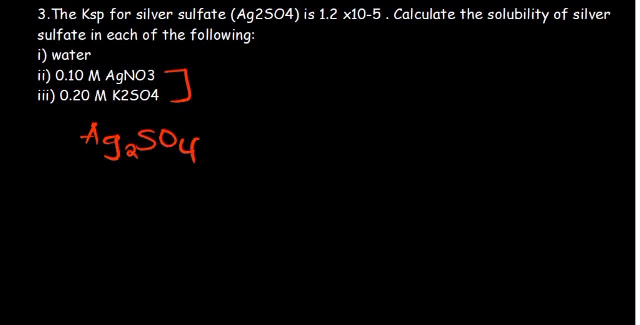 is a solid, so we've given us a KSP for the silver sulfate. so if we write our equation there, this is going to be silver and then sulfate. so what have I told you about the balancing part? so sulfate moves as it is, so it seems there is just a 1 there. 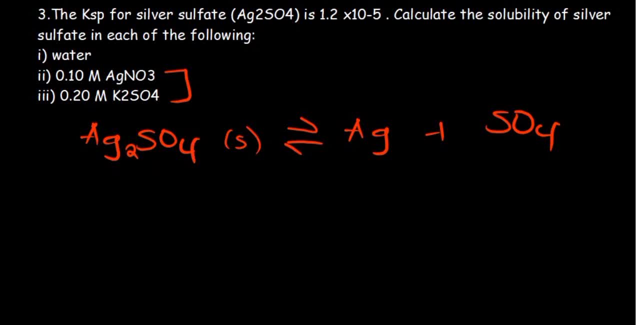 as a coefficient right as a subscript, sorry so. therefore, therefore, it tells us, silver is a plus, and then this stall go vào as a minus for a sulfate 2 minus. so therefore we have Ag plus, sulfur 2 minus, and then silver, we have 2. 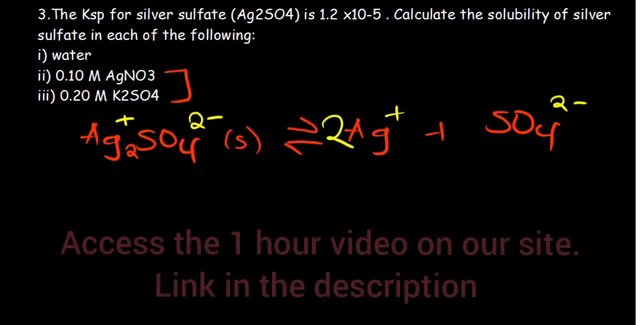 because is subscript, so I put a 2 there. so we've balanced our equation there. of course, only the right hand side, what we have is in aqua state. so we didn't even ask for us to write the dissolution reaction. so so, even if you don't show, ob'id, no. 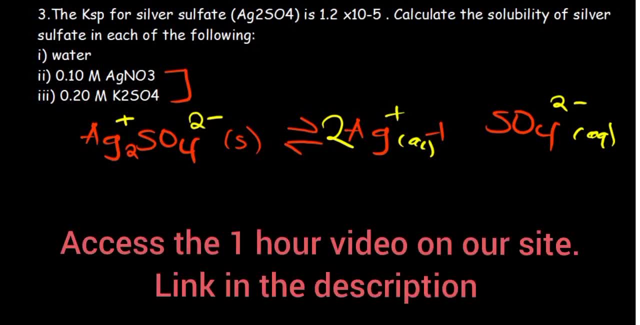 problem there. Now we need to calculate the solubility. What have they given us? They have given us the KSP. The KSP value has been given And, of course, if you try to draw up your ice table, If you try to draw up your ice table, So grab a pen, copy this ice table. 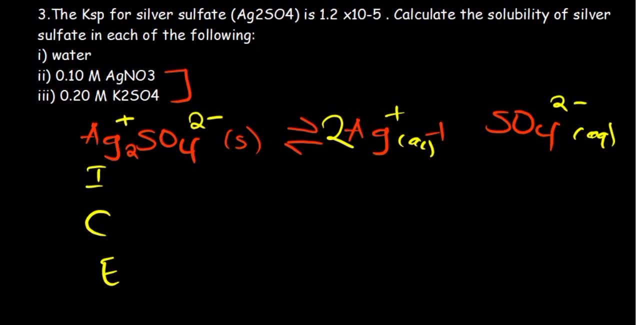 and copy for the other two so that you will be able to see the difference that is there in terms of the presence of the ions, So where we have water, Of course. in every case, we don't consider the solids to be part of our K expressions, So we didn't have any initial 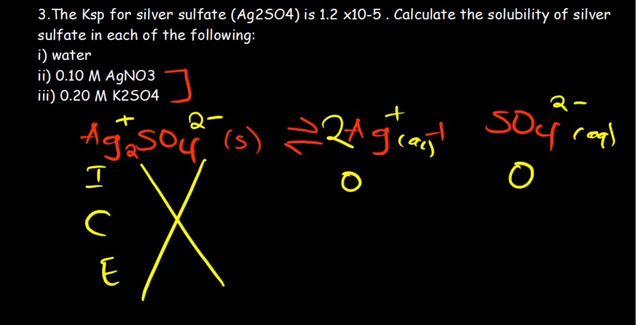 concentration of any ions in water. We just put zeros for the initial And then our change was going to be dependent on the coefficients. So plus 2X because of the 2 and then plus the 1 because it's just a 1 for the sulphate there. So therefore our equilibrium will. 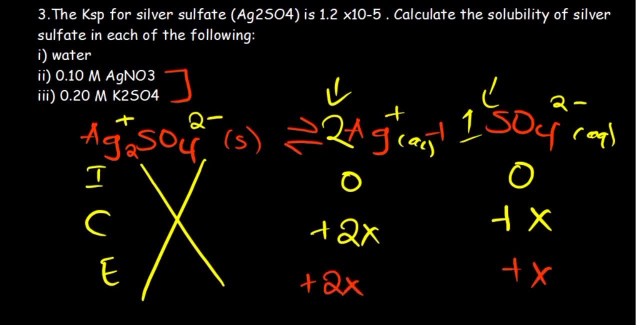 remain 2, X because of the韓heid. So therefore our equilibrium will remain 2 X, x and x respectively. writing our ksp expression, it's going to be 2x to the power 2 and then x to power 1. so raise the equilibrium concentrations to the coefficients in the equation and that's. 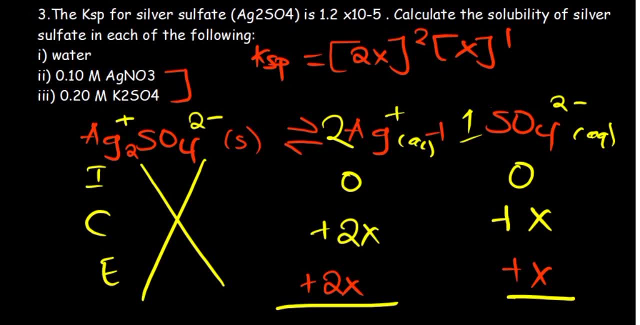 what we've basically done. so that is our ksp expression. so our ksp is going to be: 2x squared is the same as 4x squared times x, which is going to be 4x to the power 3.. okay, so allow me to now. 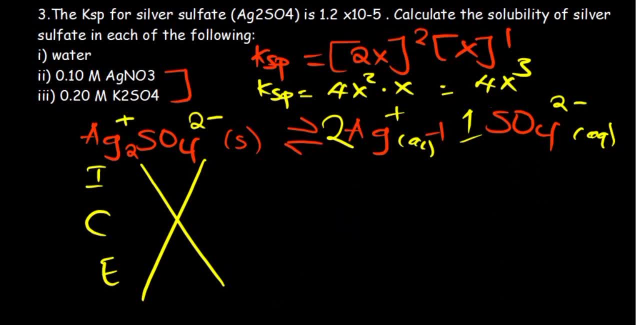 uh, clear this part to just help me simplify everything. so our ksp is equal to 4x to the power 3.. now we do know that x denotes what the solubility that they want us to find. so all you have to do is just substitute for the ksp, because the value has been given. 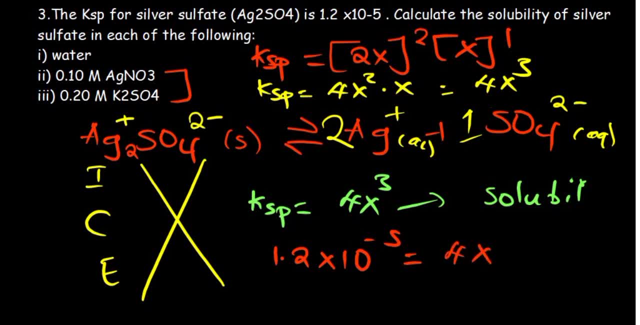 and then we are trying to find the value of what, the value of x. so divide by 4 on both sides. after that you can agree with me that on the right hand side they're just going to remain with x cubed. so you'd want to find the fades or the cube root- sorry, the cube root of. 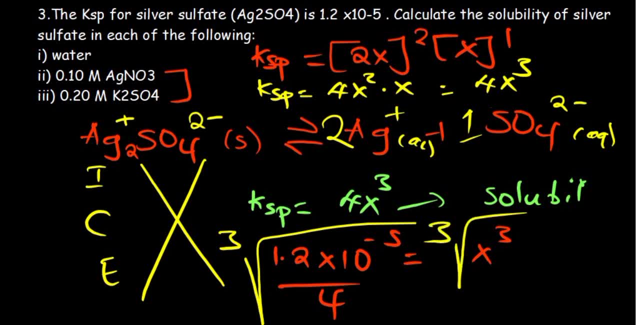 of both sides, so that your value of x is going to be determined. so let me just punch that 1.2 by 10 to the power negative 5, divided it by 4, and then we're trying to find the third, the cube root there.